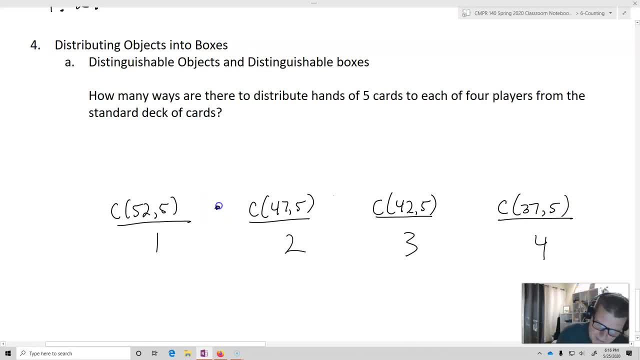 So that's the one player that's going to have 42 cards remaining, okay? Then, since we've got the four players, we're just simply going to multiply all of them together. What this is going to end up giving me is it's going to end up giving me- it's going to be 52 factorial okay divided by five factorial okay times 47 factorial right. 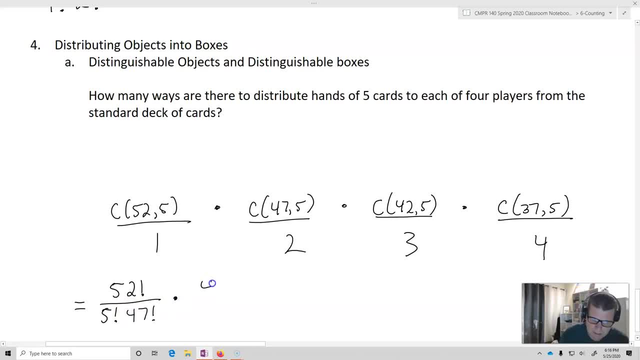 Remember, that's a combination, That's how we do them, But then 47 factorial divided by- and this will be 5 factorial for the five cards divided by 42 factorial, right, these two have to add up 47, which they do. 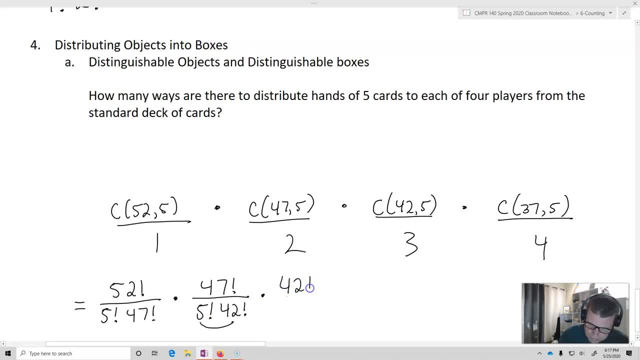 multiply it by 42 factorial now for the 42 cards that we could choose from, divided by 5 factorial, divided by, in this case, 37 factorial okay times, and this will be 37 factorial divided by again 5 factorial okay times: 32 factorial for the 32 cards that we now have left over. 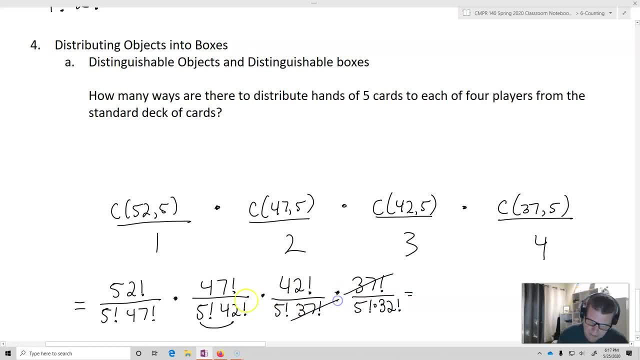 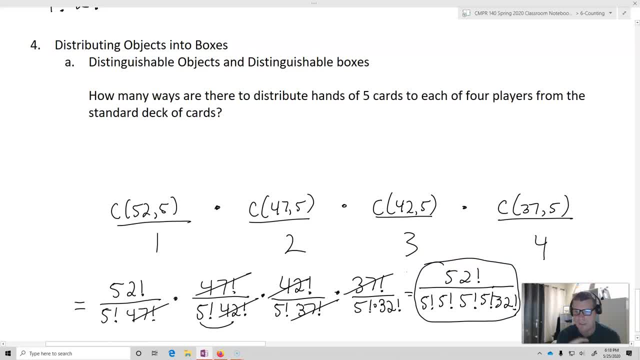 going to happen when we have distinguishable objects in this into distinguishable boxes? okay, and we're going to cancel, okay, and what we're left with is 52 factorial divided by right. we've got the total number of objects that we're going to be actually distributing. 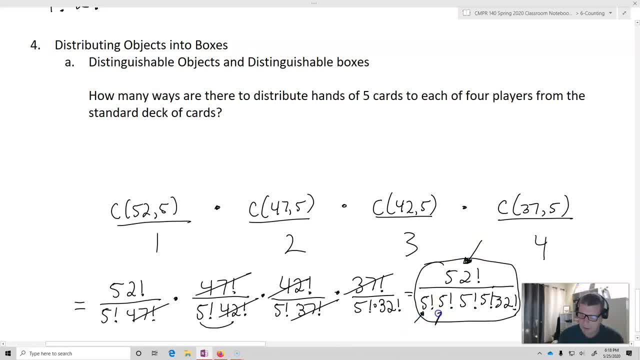 we're going to divide by how many we have in each one of the boxes- okay, factorial- for all the different ways that we can order them, and then divided through by all the different ways that we can actually order everything that's left over. so the idea here is is: 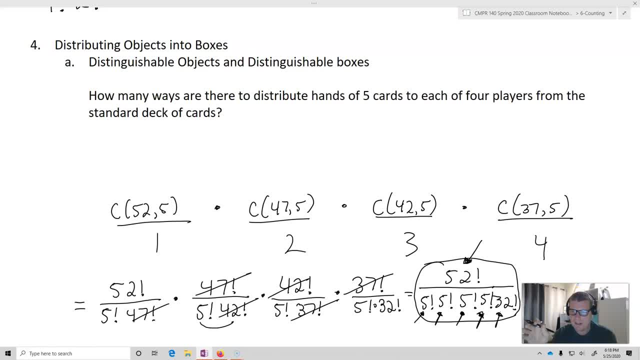 that we've placed five objects into each one of the boxes, okay, right, and each one of the elements inside of the boxes can be fact, uh, can be, uh, ordered in a certain way. hence the five factorial. but then also we've got the 32 left over, right, okay? 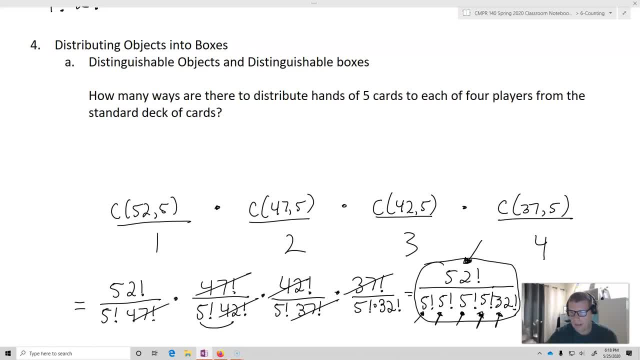 that can actually also be um ordered in a particular way, right? or has you know an amount of redundant orders as well, right? doesn't matter what's in the discard pile, if it's ace and ace spades and king of spades, or if it's king of spades and ace of spades, that order doesn't. 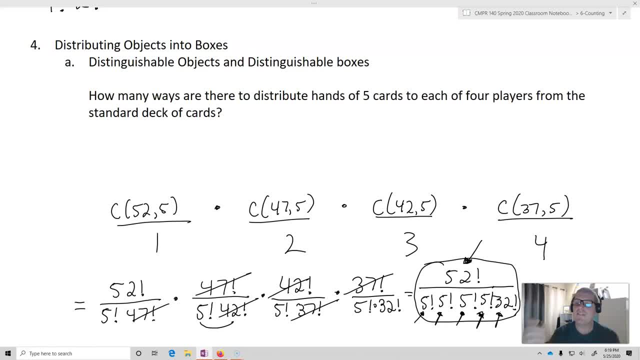 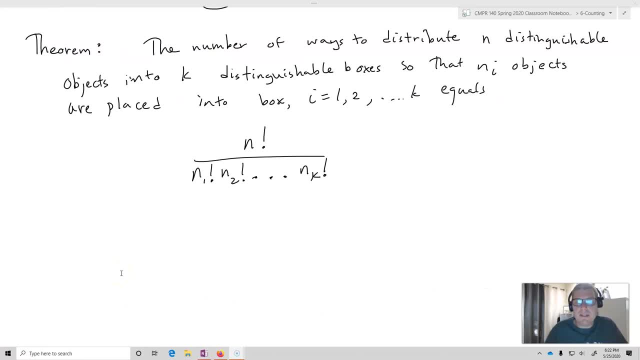 matter in the discard pile either. okay, so consequently, we've got a factor. we've got to divide out those remaining ones as well. so this gives us a theorem, and this theorem says the number of ways to distribute n distinguishable objects into k distinguishable boxes, so that ni objects are placed into the box. i, equal to one, two all the way to k equals n. 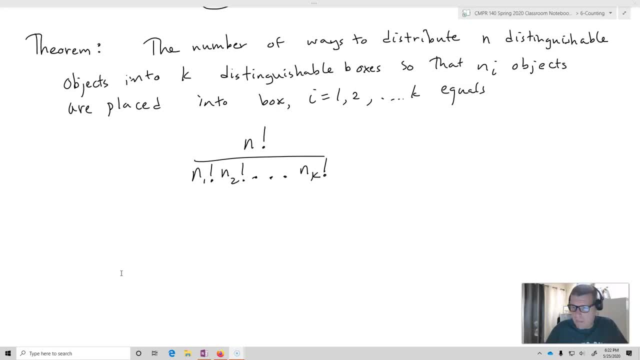 factorial divided by n1 factorial, so n1 being the number of objects in the first box and two factorial being how many uh objects are in the second box. all right, so let's get right down to nk factorial in our example we actually had, even though we had. 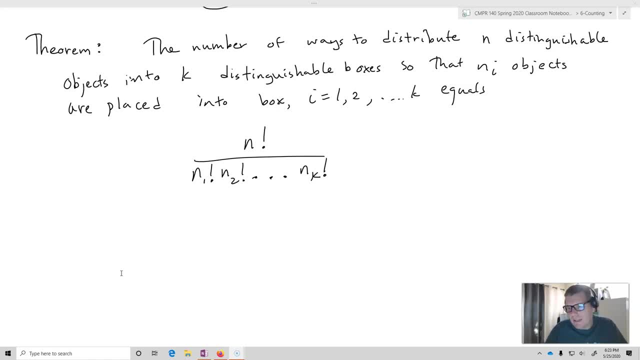 um, five players playing right. the sixth box is the discard pile. that is, all the cards that are remaining that we actually did not distribute out to any individual player. you do actually have to take into account those right and n1 through nk. okay, um, while they don't have to. 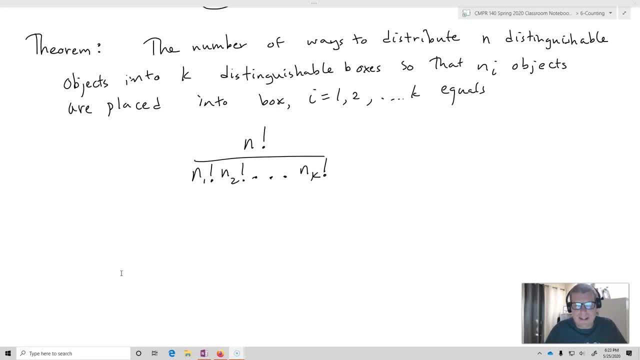 actually, uh, add up to n, right? you should consider whether or not that that's actually going to be the case. do n1 plus right? is the summation of n1 to nk going to actually equal n? in our case it did, and so we actually had to account for the fact that we had that discard pile right? let's take a look at. 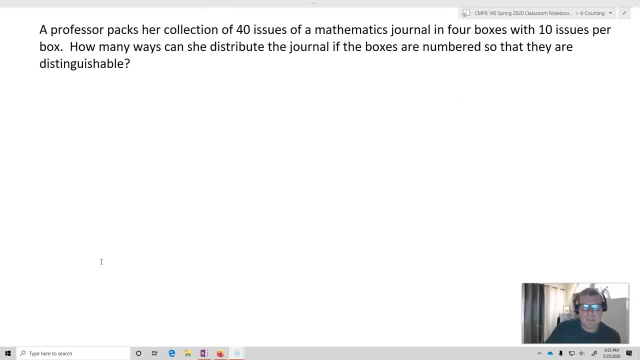 another example. so let's look at this problem. a professor packs her collection of 40 issues of a mathematical journal in four boxes with 10 issues per box. how many ways can she distribute the journal if the boxes are numbered so that they are distinguishable? so first notice, there are issues. 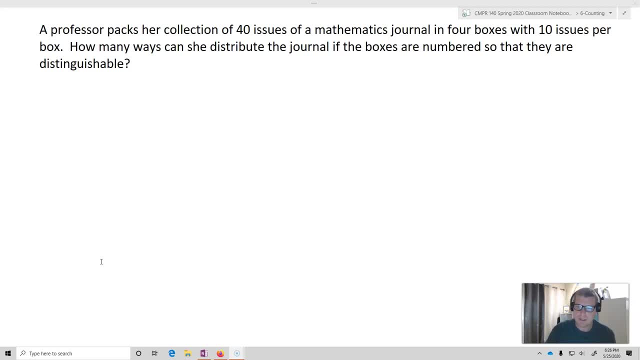 probably distinguishable. i don't know why you'd have 40 issues of the same journal. well, you know, maybe if it was like your first article, i don't know. let's just say that they're. they're distinguishable. we can tell the difference, okay, and we want to place them into four boxes with 10. 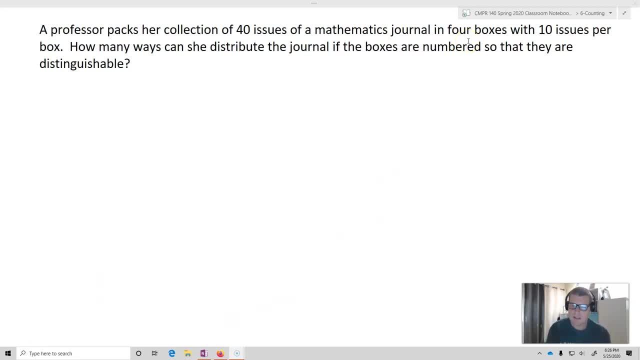 issues per box and the boxes are distinguishable. so this is: distinguishable objects into into distinguishable- uh, distinguishable objects into distinguishable boxes. okay, so we start out, we're gonna have 40 factorial- okay, that's the total number of issues, and then we're gonna have 40. 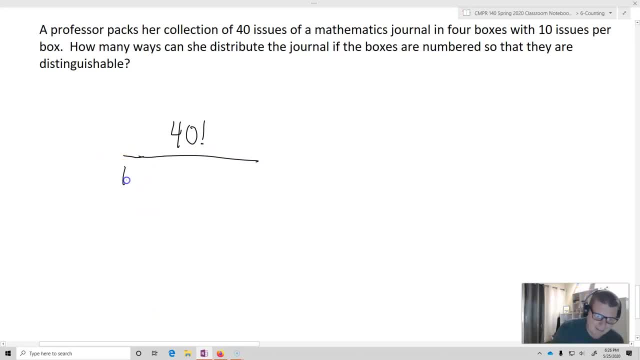 factorial, and then we're gonna divide out, right, 10 factorial for each one of the boxes, right, and there we go. that's it, 40 factorial for the issues, the mathematics journal, and then we'll divide out the 10 for the ordering of each individual set of 10. okay, that's our answer. 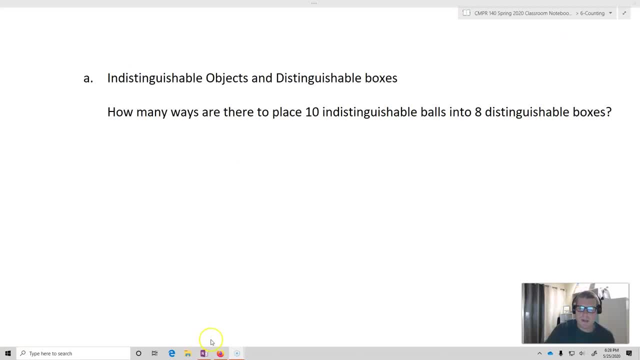 so now the next set of problems are working with these indistinguishable objects and distinguishable boxes, and we're going to divide out the 10 for each set of 10. okay, and then we're Now. what we're going to use to do this is we're going to use the stars and bars again, right, 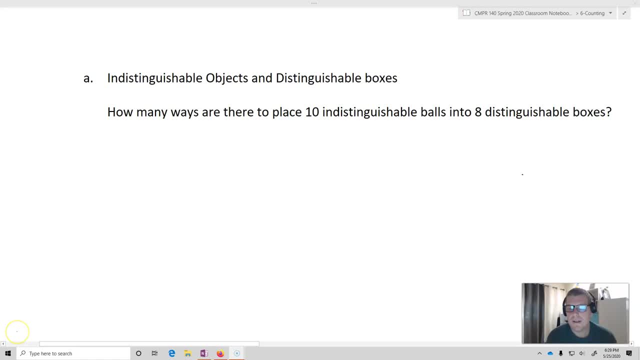 You're going to see why in just a second It actually works out really well. So let's suppose that I have this question. This question is: how many ways are there to place ten indistinguishable balls and eight distinguishable boxes? So I'm going to use stars and bars here. I'm going to have box one. 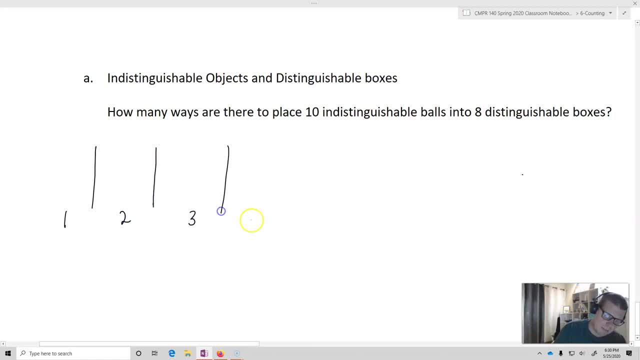 box two, box three, box four, box five, box six, box seven and then box eight. I don't need a line for box eight- And there are all my bars. Then I'm going to place my ten distinguishable balls. Let's say, for example, I put three into two. 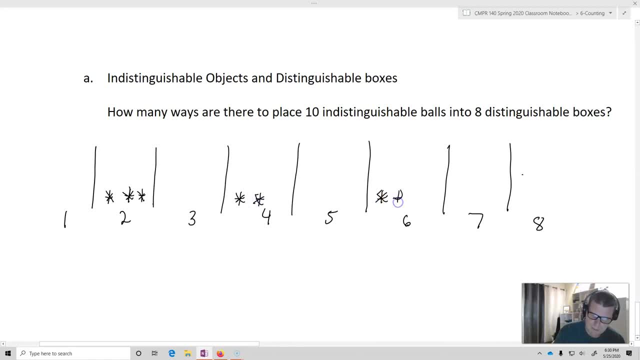 two into four and five into six. okay, What I've basically done- five into six, what I've basically done here, or more than basically, is I've said: okay, you know what I've got For each one? for each one of the bars, I've got a slot, and each one of the stars, I have a slot. 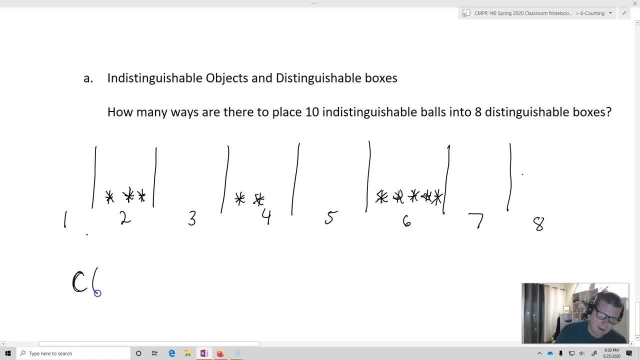 So I have, I'm going to do a combination of, in this case, eight plus ten minus one, and I'm going to choose slots for one, two, three, four, five, six, seven, eight, nine, ten.